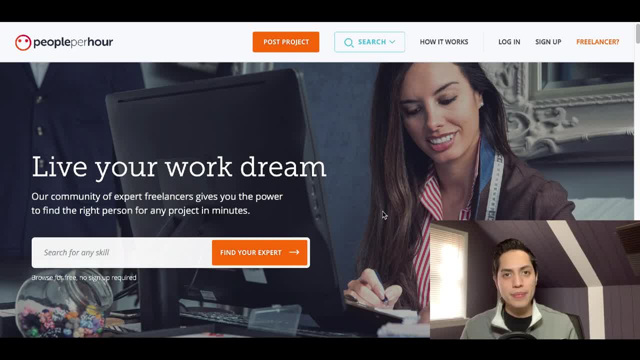 create videos. you can come on here, create your own profile and people can hire you to become a freelancer for them. so to make their video for them, or to write an article, or write a paper for them, or do mathematics for them, start solving math problems for them. so all they would have to do 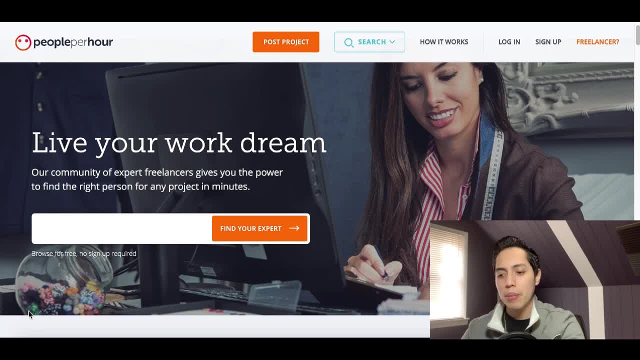 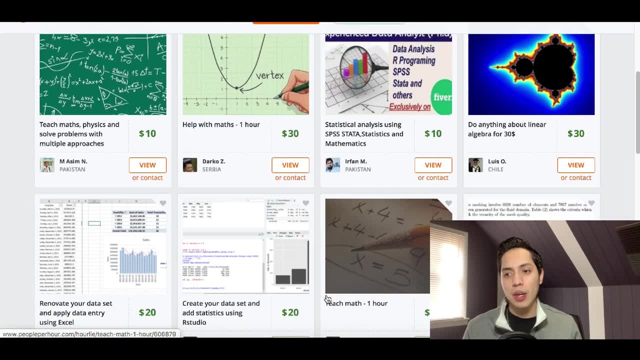 is come to people per hour inside of the search bar right here, type in mathematics. after that, all they have to do is click on find your expert and they're going to see a whole bunch of different profiles of people that can help them out with their math problems. so, as you can see right here, 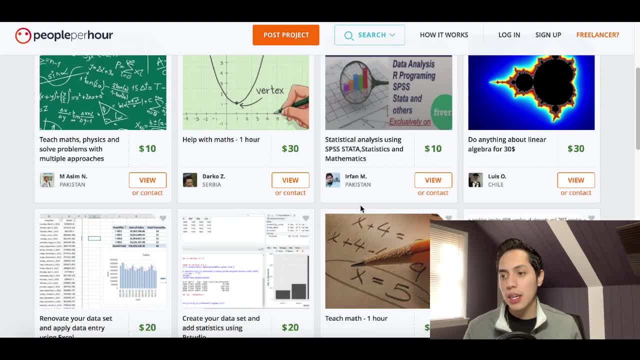 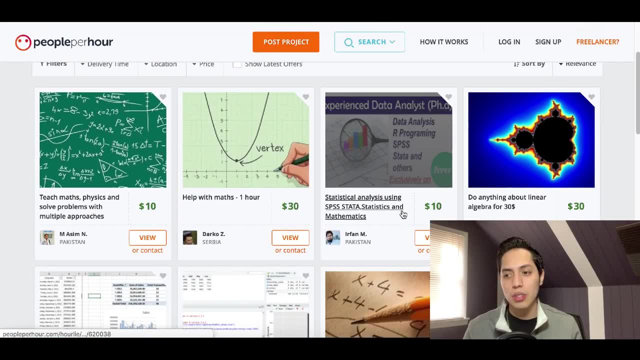 they're going to start seeing profiles of people that can actually help them with their mathematics. this guy charges 10 bucks per hour, 30 dollars per hour. they'll start seeing profiles of people that can actually help them with their mathematics skills. so all they have to do is click on one. 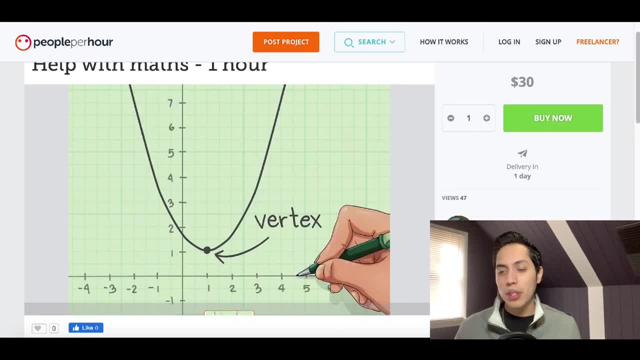 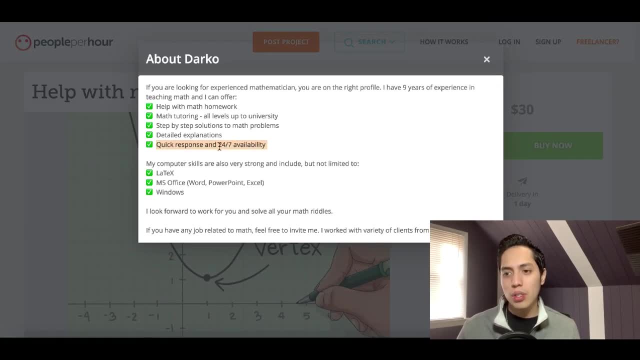 of these profiles right here and they could start seeing more information about the person's profile, so, for example, obviously his name and more about what he does right here. so he's been. he has a quick response, usually available 24 hours. the math tutor all levels of university and you know step. 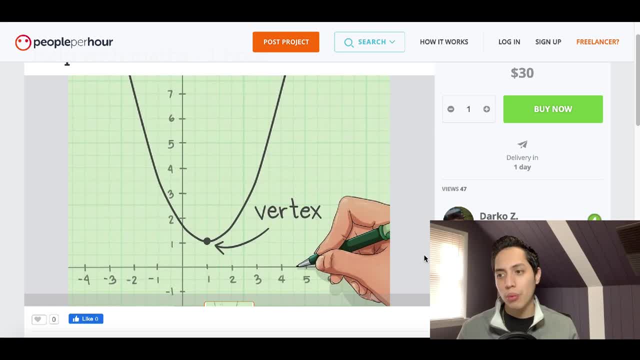 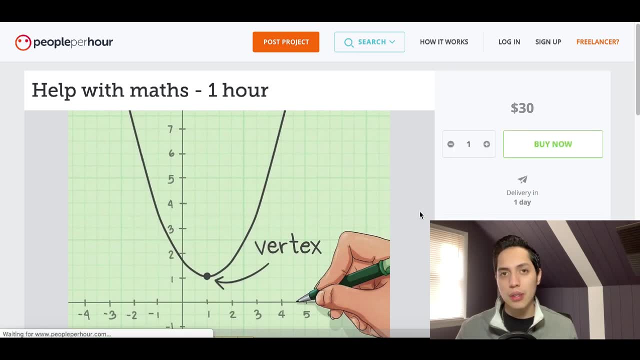 more information on the person, their job, exactly how things are going to work, and once they're ready to hire them and, you know, get the job- all they have to do is click on buy now and they can go ahead and get started with this. so what you want to do to start making money solving math? 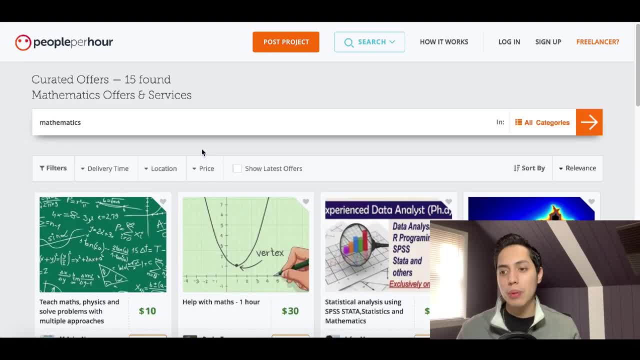 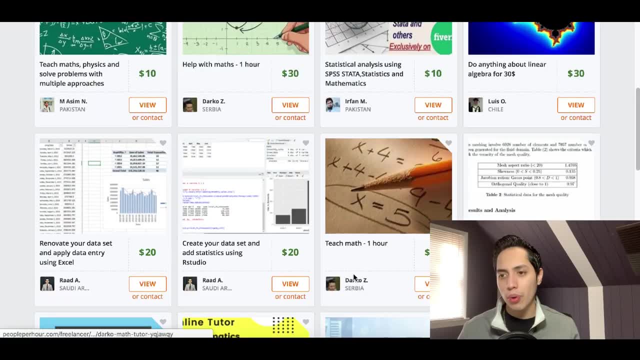 problems is create your own people per hour profile, just like these people have right here and, as you can see right here, check this out. there's not a ton of people doing this right now. there's an overall maybe about 12 or 13 profiles, so you can be the next one by creating. 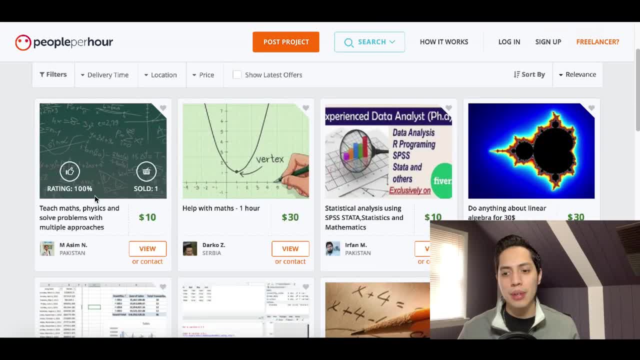 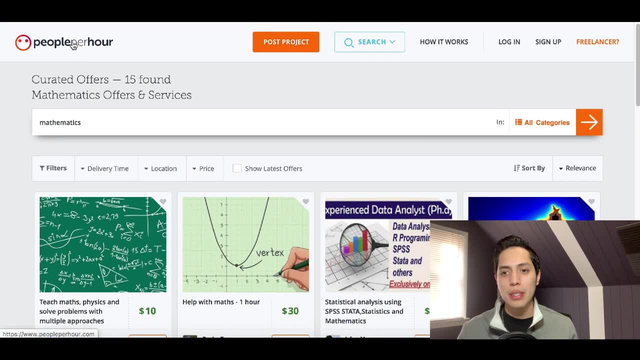 your own profile and start offering your services on people per hour again, you can charge anywhere between 10 or 30 dollars per hour just to help them solve math problems. so to sign up, just go back to the home page right here, go to the top right hand corner. 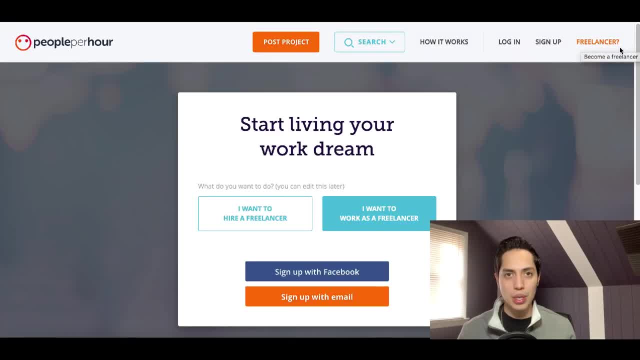 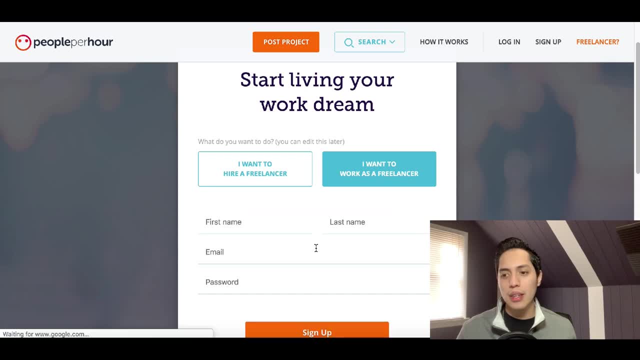 and click on become a freelancer- right here, where it says freelancer, with a question mark after that. click on i want to work as a freelancer. and sign up using your email or your facebook account. that's fine, right there, and all you're going to do is just go ahead and fill out your. 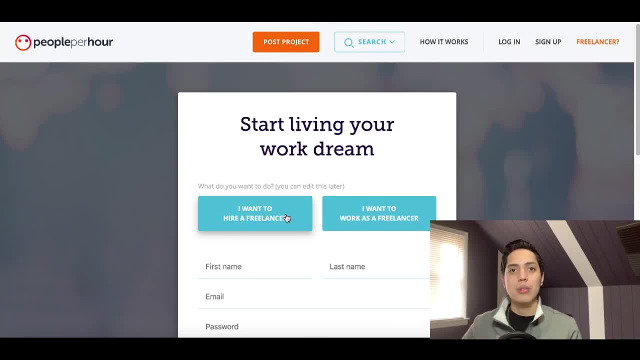 name, fill out your email and after that, you're going to start the application process to create a people per hour profile. and so, as you're filling out your application, you're going to specify the exact work you want to do on people per hour- so, obviously, helping people with math, a math tutor, and once you go ahead and submit the application, one of their 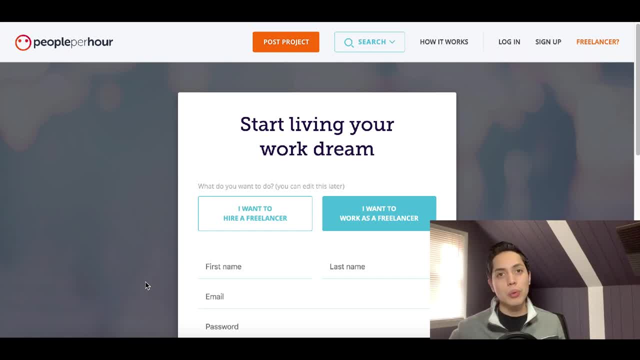 moderators is going to review and approve your application. once you're approved, you can go ahead and create your profile and start taking any job that comes your way inside of your back office. you can also submit jobs or, you know, request jobs that are inside of the back office guys. so it's an easy. 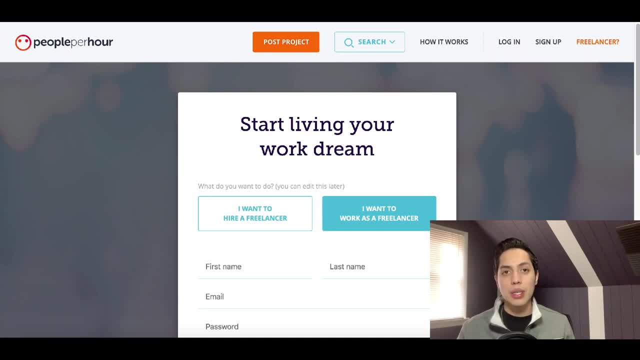 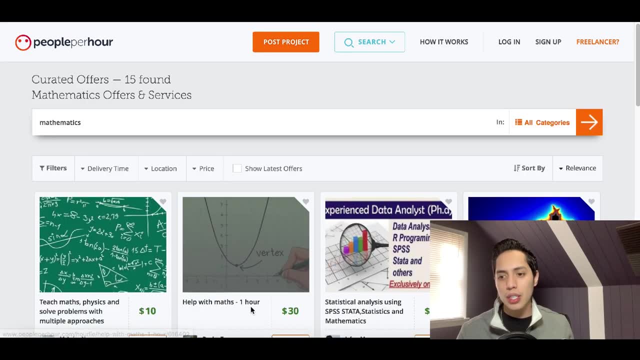 way to start getting more jobs inside of people per hour. now, the trick to getting more jobs- and you know, getting more work on people per hour is to start. getting more jobs inside of people per hour is really developing your profile. so if we go back over here, you're going to see that this person 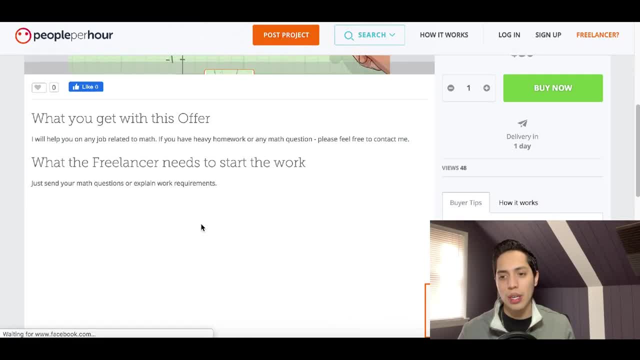 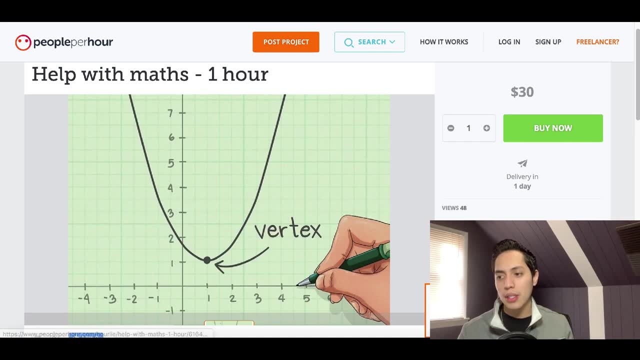 right here obviously doesn't have a ton of development with their profile. you know it has two little lines right here, doesn't even have many pictures. so you really want to make sure you develop your profile, you know, adding a lot of details as much as you can of what you're going. 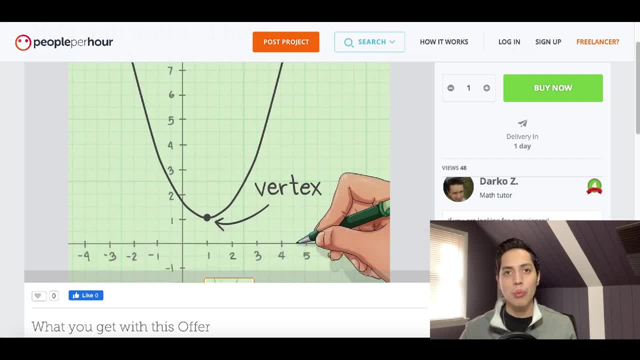 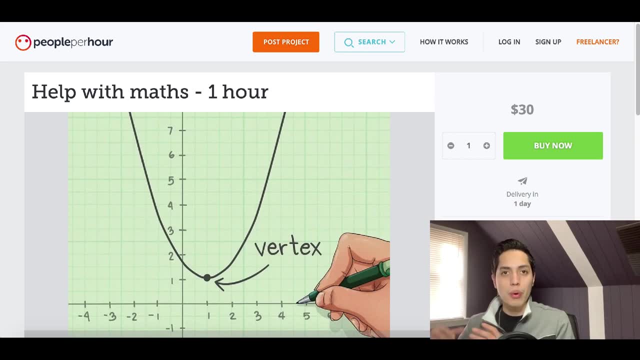 to be doing on the job. you know that way people get a better idea on what you can do, what you can actually help them with, and they're going to want to hire you more. you know it's more likely that they actually hire you someone that has a more professional profile, as opposed to someone that 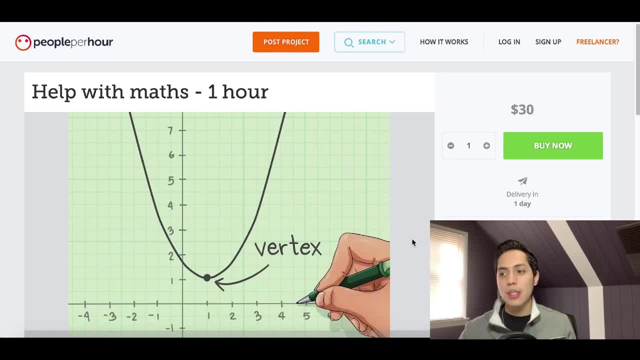 has a few little details here and there, you know one single picture. so you definitely want to make sure you add in as much info as you can to your profile so people can get a better idea on what you can help them with, which will give you a better chance to getting hired now, once you go. 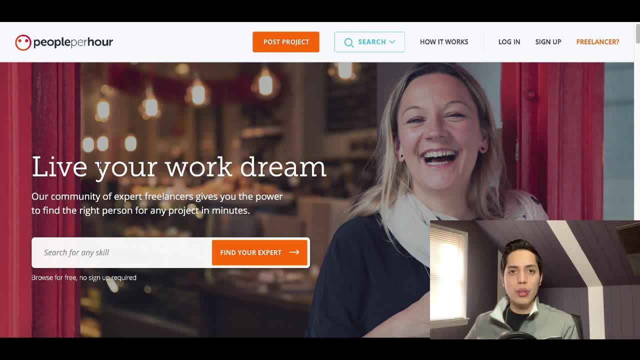 ahead and get hired for a job. what's going to happen is the buyer, or you know your client- is going to make the payment to people per hour. people per hour is going to hold on to the payment and their escrow once you complete the job and you help them out with their math, or you know. 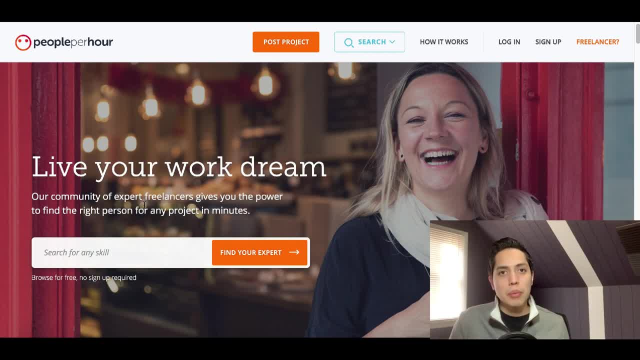 you complete the job overall people per hour is going to go ahead and release the payment to you. your account, now that's after the person that you know, after your client has approved the job. you know if you do good work and you know they like the job that you did, they're gonna go ahead. 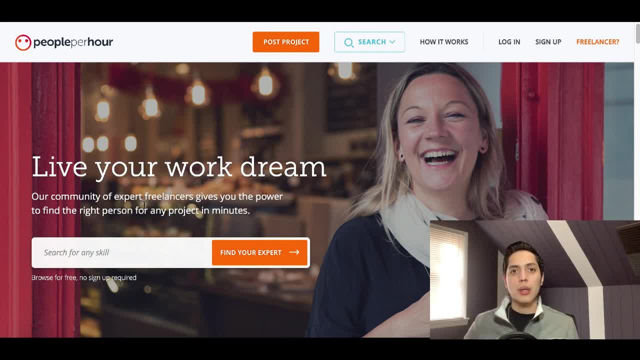 and approve the payment. after they approve the payment again, it goes into your people per hour account, which later on you can go ahead and redeem using your paypal account, using a pioneer account or using your own bank account. the payment method is up to you. you have three different options. 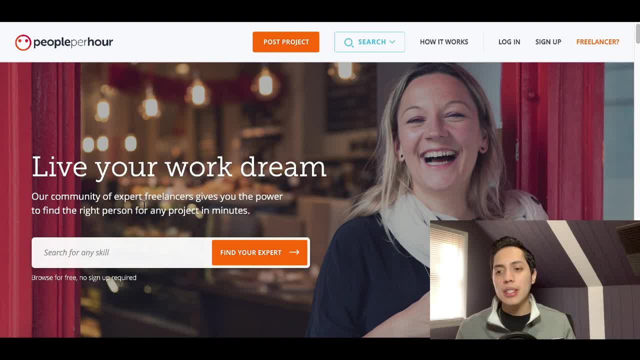 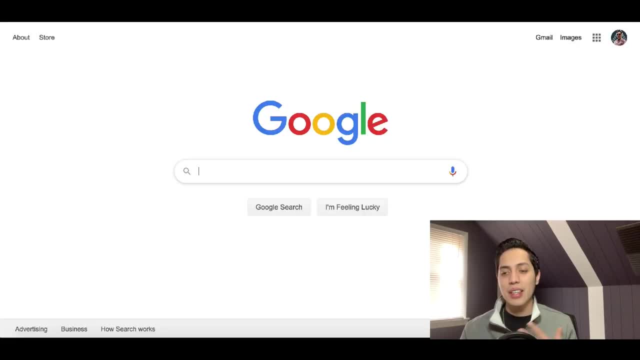 paypal, pioneer or your own bank account. so again, it's really easy to do, guys: just come on people per hour and create your own profile. so that's website number one. excuse me, i'm running out of breath a little bit. that's website number one. website number two is called fiverrcom, guys. 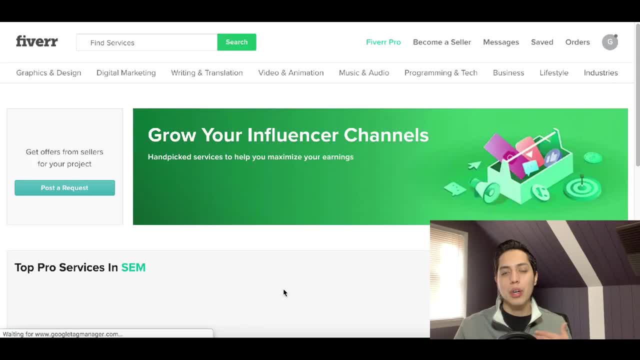 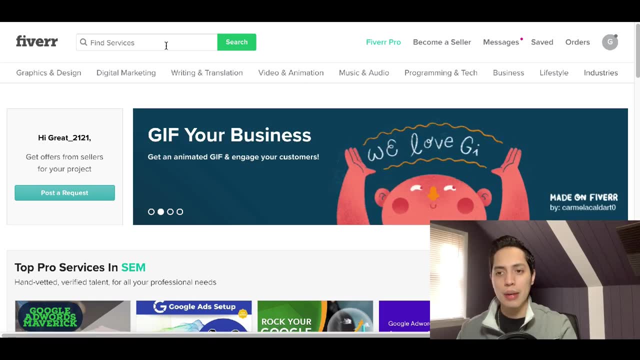 and it's basically the same thing. it's another freelancing website where you can come on here, create your own prop profile and start, you know, accepting jobs to help people with math. so all someone would have to do is come out of fiverrcom type in mathematics and after that, 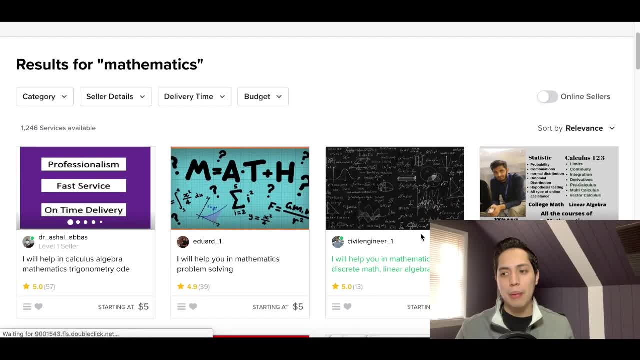 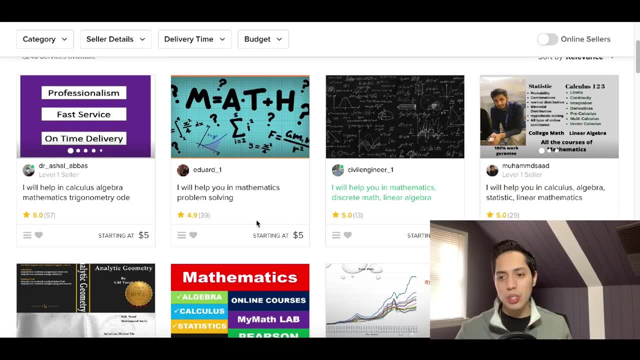 you know, different profiles of people that can actually help them with their math will pop up. you have to do is create your own profile. sign up to fiverr, create your own profile, and your profile will pop up right here, just like all these other people's, and you can start. 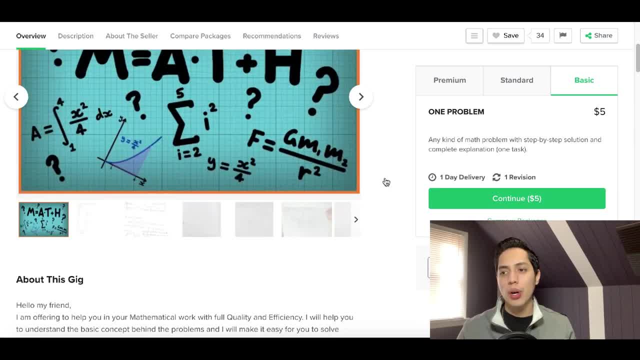 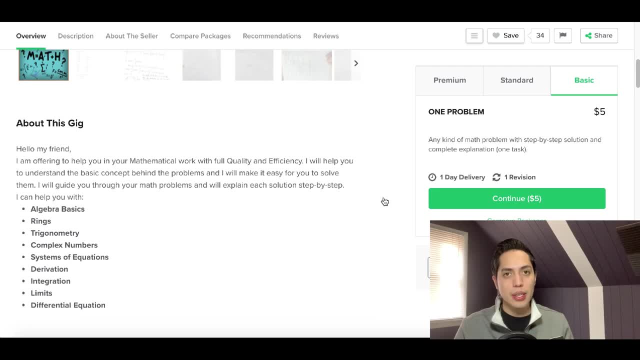 accepting any job that comes your way. again, the key point here is to go ahead and develop your profile, making sure that you know your profile stands out amongst other people. that's what's really going to make you. you know, help you start getting more jobs as a freelancer. 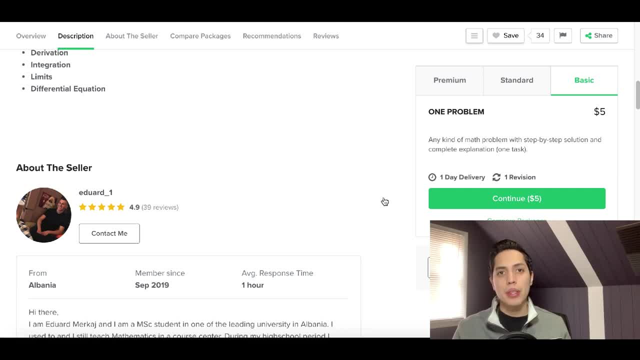 and it works the same way. once somebody hires you for a job, they're going to submit the payment. fiverr holds on to the payment in their escrow. once the job has been completed, they release the payment to your account. now, with fiverrcom, you want to make sure you do ask for a review. 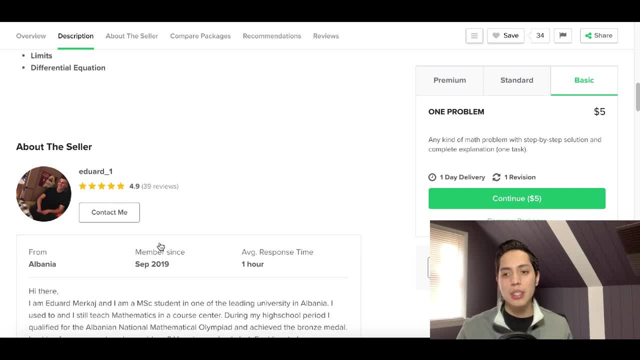 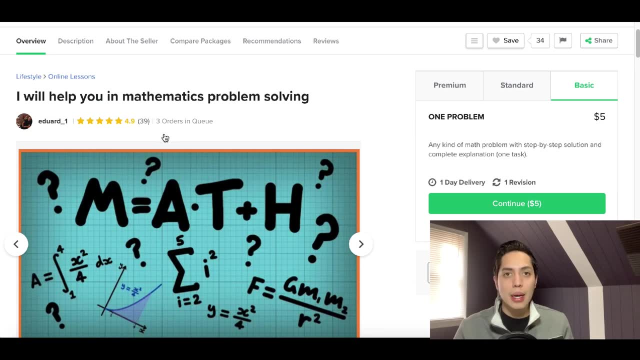 after you complete the work. after you complete the job, because obviously reviews really matter a lot. you know, when somebody new comes and checks out or someone's profile and they have, you know, close to a five-star review, it's a lot more likely that they hire them for a job. now, one thing i like: 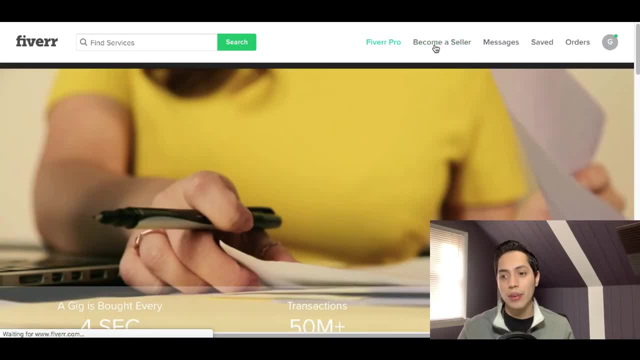 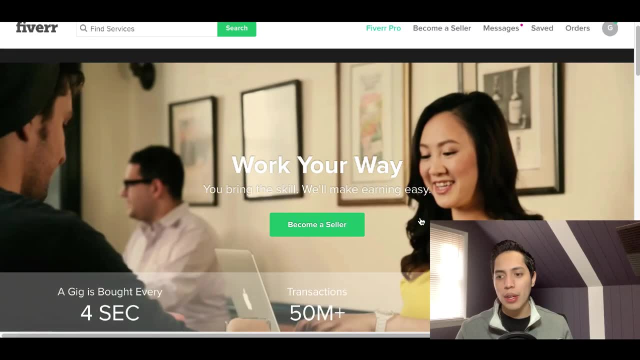 about fiverr is. that kind of gives you a better basis on building your profile right. so, if i click on, become a seller right here. so if you want to start, you know, create your own profile and start doing these type of jobs, click on, become a seller right here. you can get some. 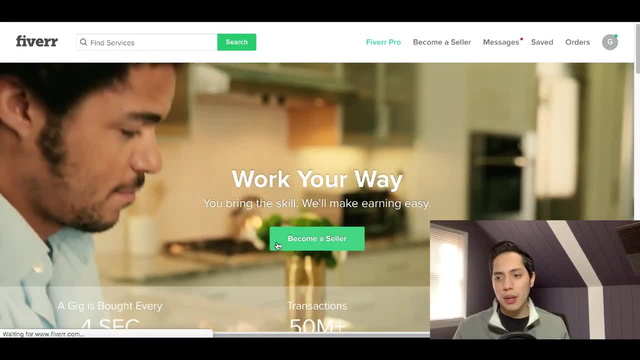 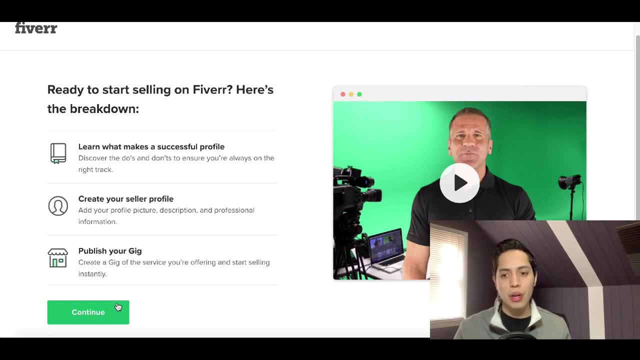 information if you start scrolling down, but go ahead and click on become a seller. after that it's going to take you through. you know, filling out your application exactly what you want to be putting on your profile to start getting more gigs and more jobs. so click on: continue, you know. 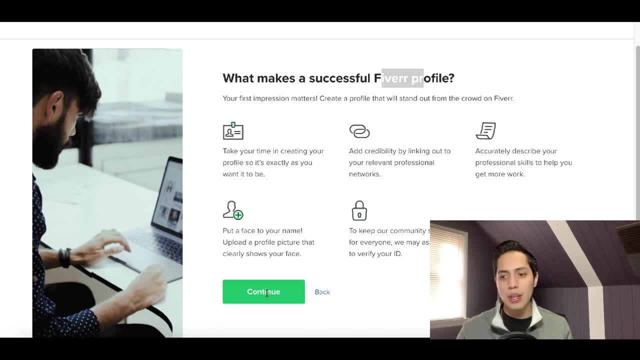 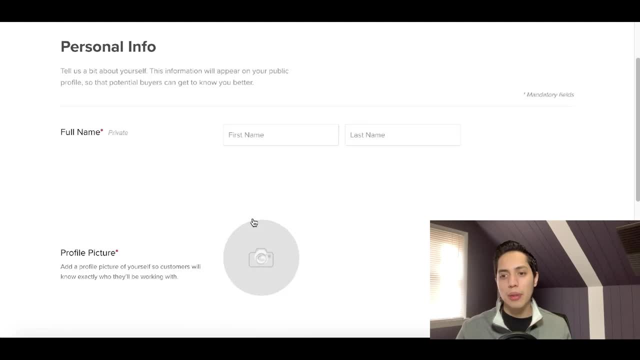 overall gives you a lot more information on building your fiverr profile. then you know exactly what you should start putting on it. then you know how to start standing out from other people's profile. so continue that with that right there and then you can get started with the. 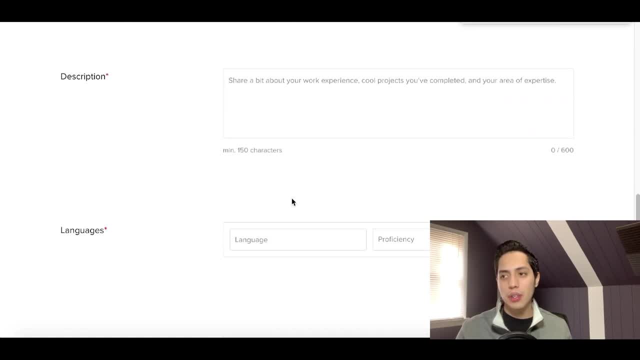 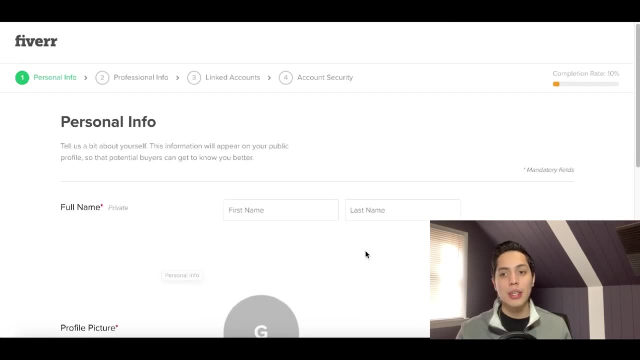 application process right here. just fill out your name, add a picture of yourself right here, you know, add in a description of who you are, exactly what type of work that you do, and just your languages. click on continue and you can go ahead and get started with the application process to create your profile. guys, so that's an easy way.